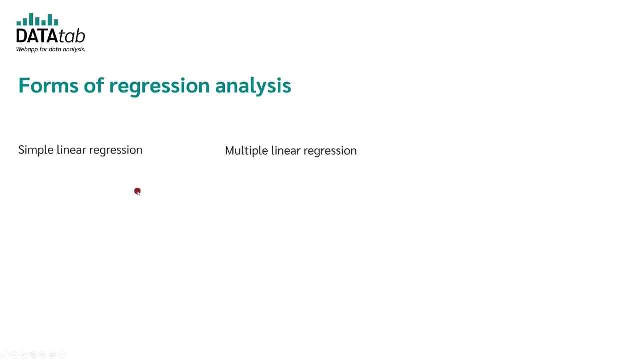 by one or more other variables. The simple linear regression uses only one independent variable to predict the dependent variable. In the example where we want to predict the salary of a person, we use a variable to predict the salary of a person In the example where we want to predict. 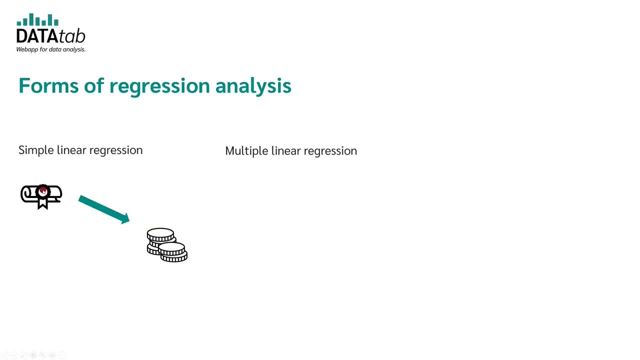 the salary of a person, we use only one variable, either whether one has started or not, the weekly working hours or the age of a person. In multiple linear regression, several independent variables are used to predict the dependent variable, So we could use the highest educational level. 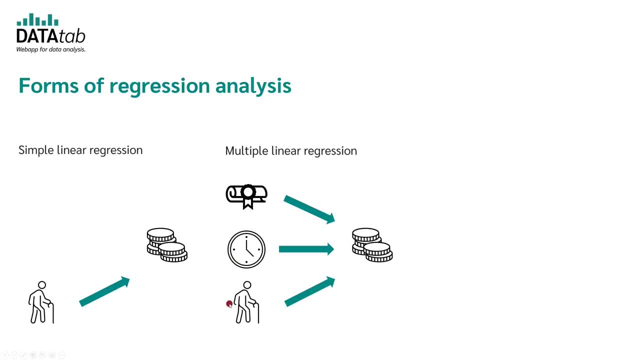 the weekly working hours and the age of a person. So, therefore, the difference between a simple regression and a multiple regression is that in one case, only one variable is used to predict the dependent variable, So one independent variable is used, and in the other case we use several different independent variables. 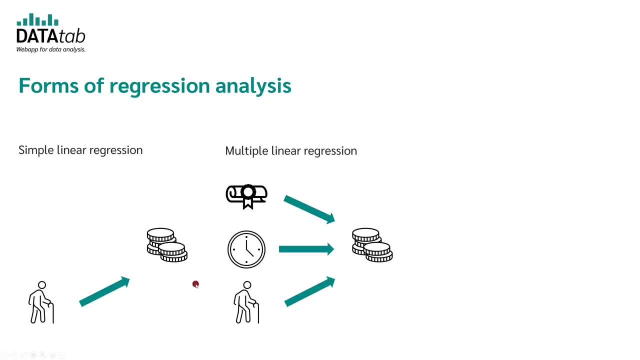 Different Results. Both forms of regression have in common that defined variable is metric and a metric variable For example, the salary of a person, the body size, the shoes, eyes or the electricity consumption. in contrast to that, the logistic regression is used when you have a categorical dependent variable. Logistic regression data include them this way as well. 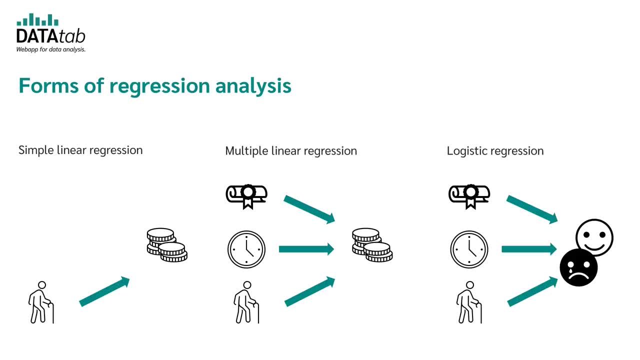 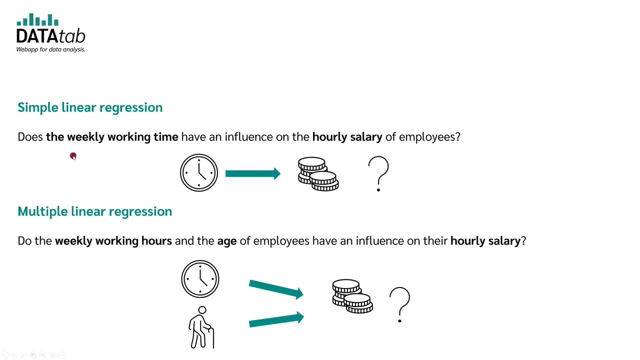 regression is discussed in a separate video in this playlist. So let's summarize the information. The simple linear regression is used for the question: does the weekly working time have an influence on the hourly salary of employees? So there's only one independent variable used, which is the weekly working time. 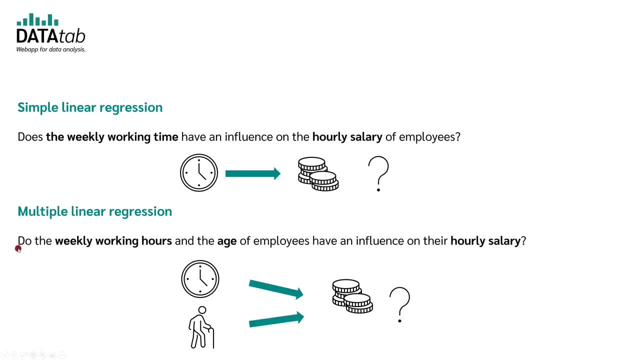 The multiple linear regression could be used for the question: do the weekly working hours and the age of employees have an influence on their hourly salary? So in this case we have two independent variables: the weekly working hours and the age of employees. Let's first start with the simple linear regression. 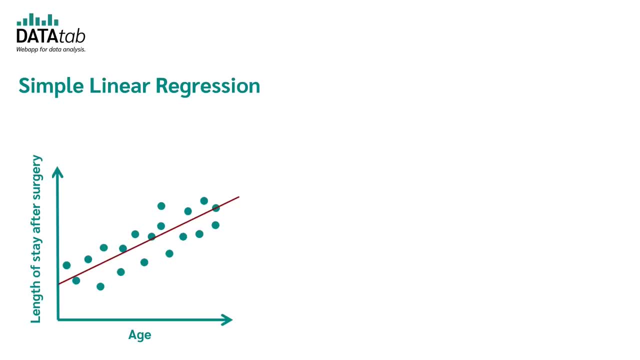 The goal of a simple linear regression is to predict the value of a dependent variable based on an independent variable. The greater the linear relationship between the independent variable and the dependent variable is, the more accurate is the prediction. Visually, the relationship between the variables can be represented in a scatterplot. 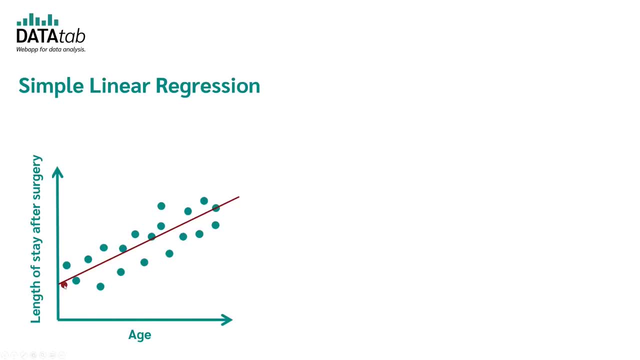 The greater the linear relationship between the dependent and the independent variable is, the more the data points lie on one straight line. The task of a simple linear regression now is to determine exactly the straight line that best describes the linear relationship between the dependent and the independent. 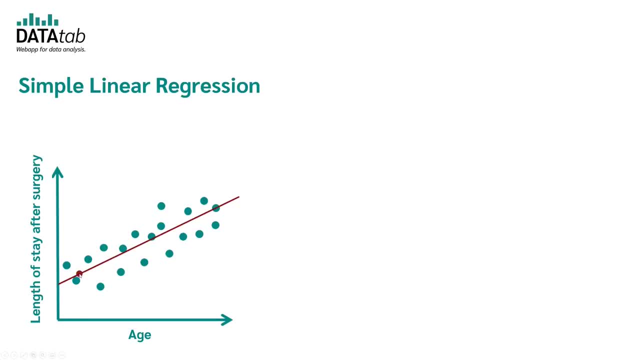 variable. In the context of linear regression analysis, a straight line is plotted on a scatterplot. To determine this straight line, linear regression uses the method of least squares. Let's say a hospital has asked you to give them an estimate based on the age of a person. 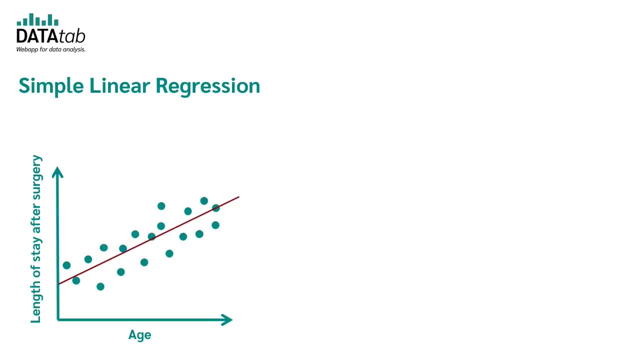 of how long that person will stay in the hospital. Let's say a hospital has asked you to give them an estimate based on the age of a person, of how long that person will stay in the hospital. Let's say a hospital has asked you to give them an estimate based on the age of a person. 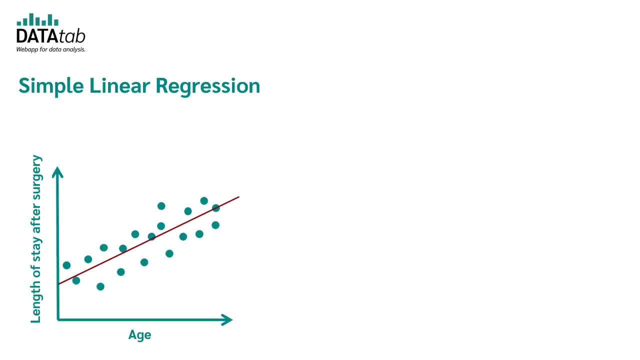 of how long that person will stay in the hospital after a surgery. Let's say, a hospital has asked you to give them an estimate, based on the age of a person, of how long that person will stay in the hospital after a surgery. With this information, hospital operators want to optimize their planning. 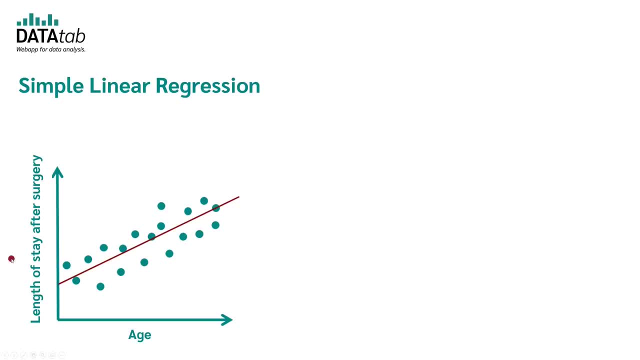 Your dependent variable, the one you want to predict, is, for example, the length of stay after the surgery, And your independent variable is age. The equation that describes the model now looks like this. So in this equation, y hat is the estimated length of stay. 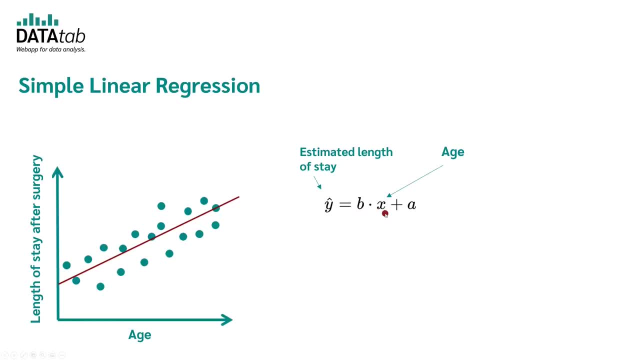 B is the slope, X is the age And A is the receptor point. So this is the intercept with the y-axis. So the receptor point tells you that if a person is zero years old, this person stays A days in the hospital. 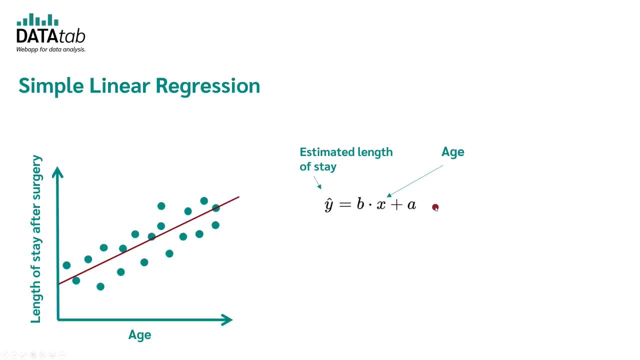 In order to calculate the coefficients, the hospital must, of course, give you a sample of people from whom you know the age and the length of stay after surgery. So with the data you got, you could, for example, find out that B is 0.14 and A is 1.2.. 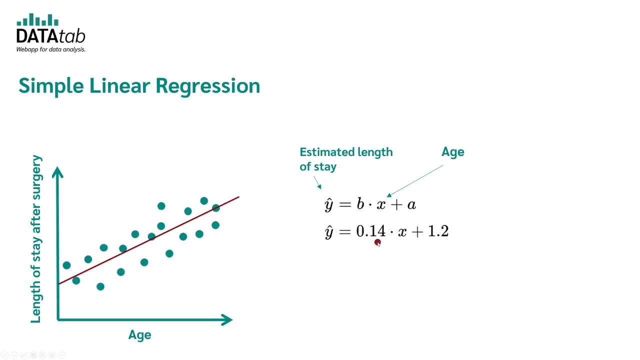 This is now your model, and with this model, you can estimate the length of stay after surgery based on the age of a person. So what does this mean? now, If we assume that there is a person who is 33 years old and is registered for a surgery, 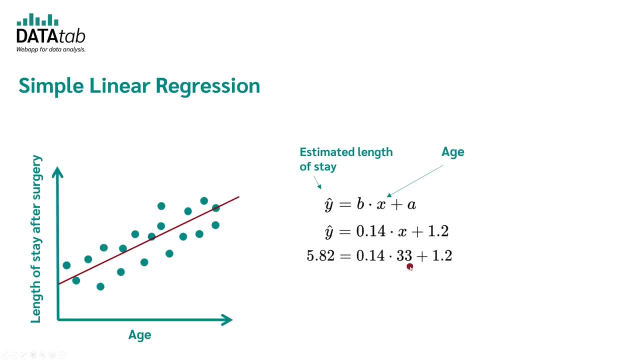 we put 33.4.. Our model then tells us that this person stays in the hospital for 5.82 days after surgery. Now, of course, the question is: how do you calculate the slope B and how do you calculate the intercept A? 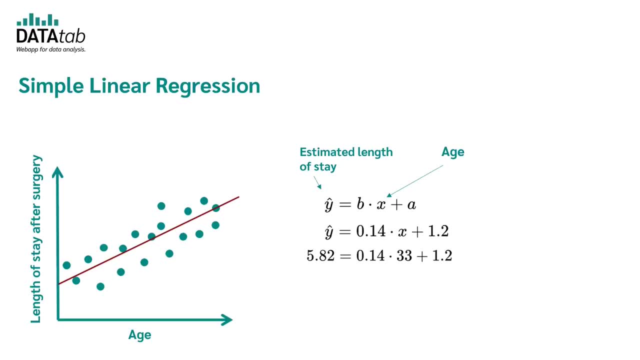 Usually you just use a statistics program like DataTab In the case of a simple linear regression. however, it is also quite simple to calculate it by hand. B results from the correlation of the two variables times the standard deviation of the variable length of stay after surgery divided by the standard deviation of age. 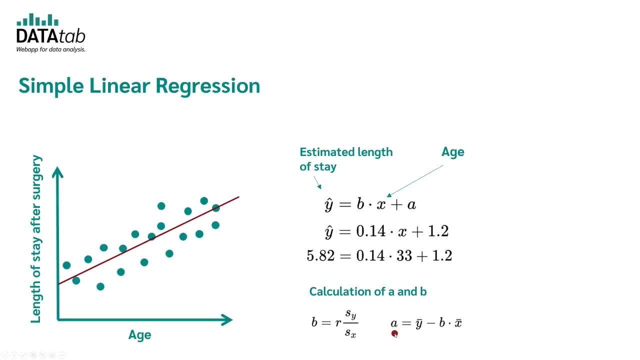 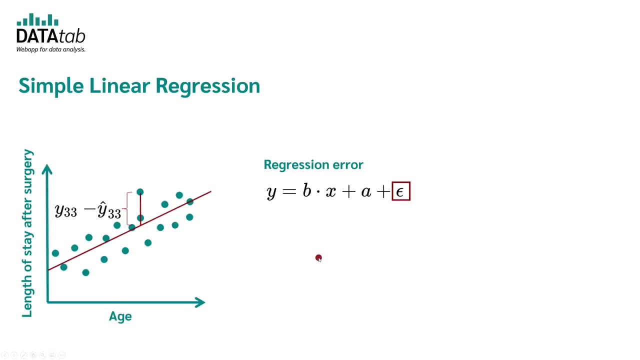 A is obtained by calculating the mean value of the length of stay minus the slope times the mean value of the age. The regression line always tries to map the given data with a straight line as best as possible. Of course, this always results in an error. 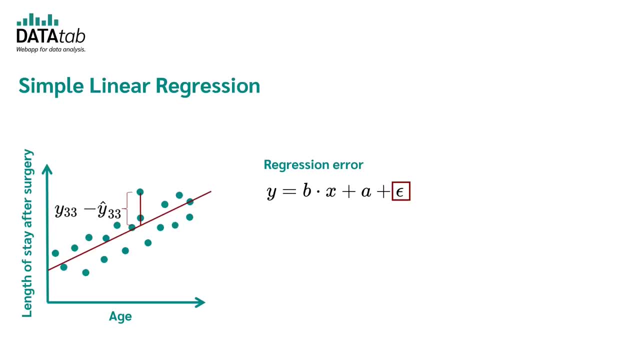 This error is called epsilon. Let's say we estimate the length of stay after surgery of a person who is 33 years old. Our model tells us that the person stays in the hospital for 5.82 days, but in fact he or she stays in the hospital for 7 days. 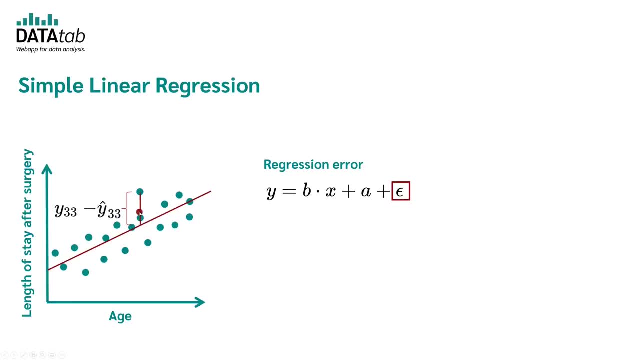 Then the difference between the estimated value and the estimated error is calculated, and the true value is our error. Now you have a good overview of what a simple linear regression is, and we come to the multiple linear regression. In contrast to the simple linear regression, the multiple linear regression can include: 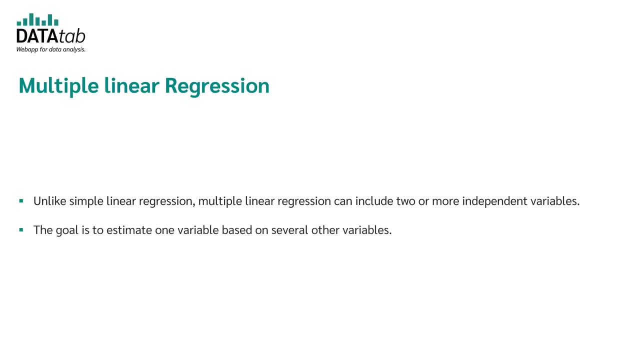 two or more independent variables. As we already know, the goal of a regression is to estimate one variable based on several other variables. The variable to be estimated is called the dependent variable or criterion. The variables that are used for prediction are called independent variables or predictors. 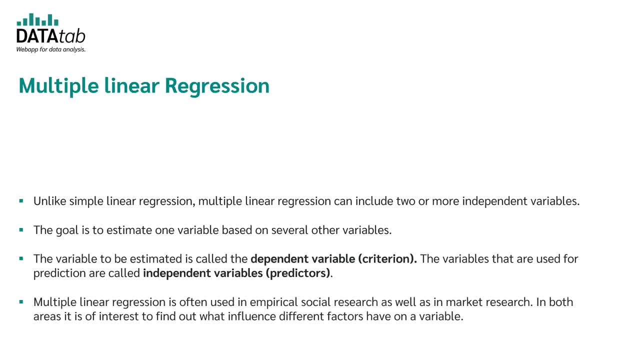 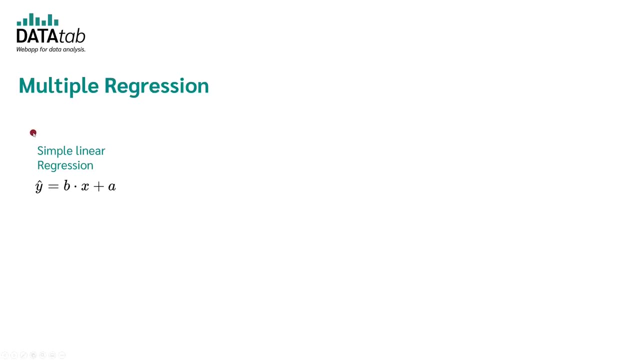 Multiple linear regression is often used in empirical social research as well as in market research. In both areas, it is of great interest to find out what influence different factors have on a certain variable. As we already know, this is what the equation for a simple linear regression looks like. 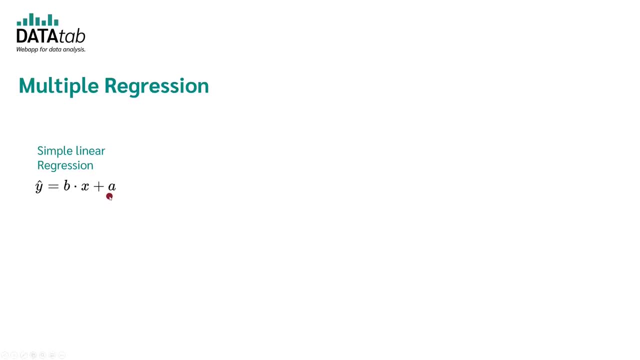 We have one independent variable, x, plus the constant a. If we now go to the way of multiple linear regression, we have several independent variables. So we have the first variable, the second variable and the k-th variable. The coefficients can now be interpreted similarly to the linear regression. 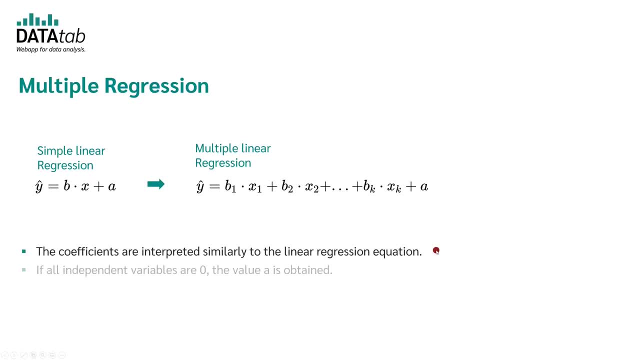 So we have the first variable, the second variable and the k-th variable. The coefficients and the k-th variables have a significant influence on the linear regression equation. So what do we do now? We change the response of the independent variable to the linear regression equation. 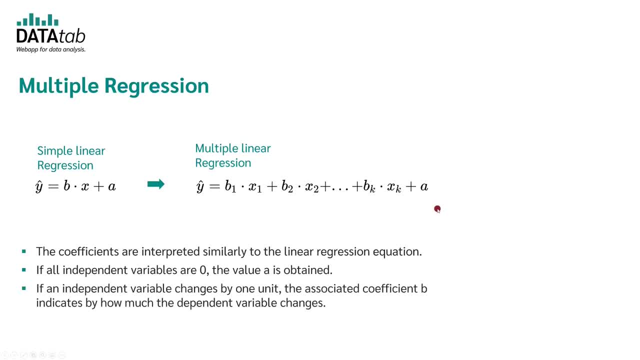 If all independent variables are 0, we get the value a. If an independent variable changes by one unit, the corresponding coefficient b indicates by how much the dependent variable changes. Before I show you how to interpret the results of a regression, I will first explain how. 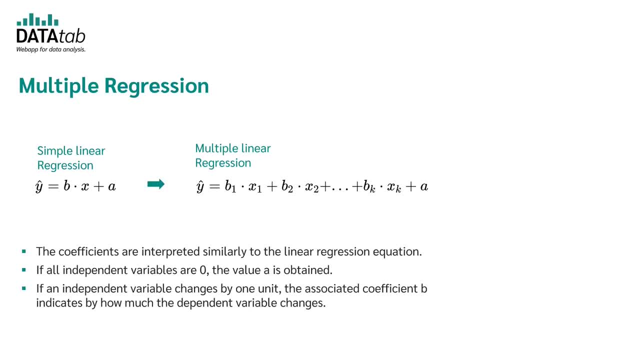 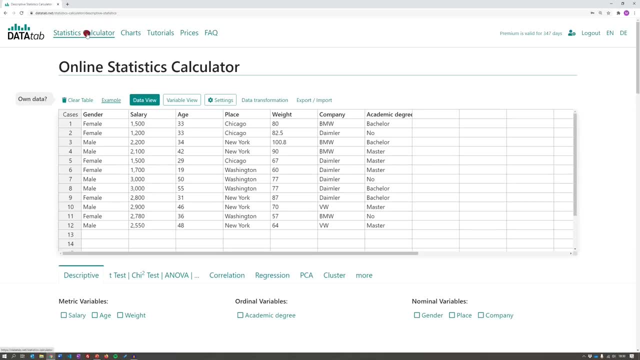 you can easily calculate a linear regression online. How to interpret a linear regression online. to do this, please visit datadapnet and click on the statistics calculator. If you want to use your own data, just click on clear table. I'm going to use the example data now. So now we want to. 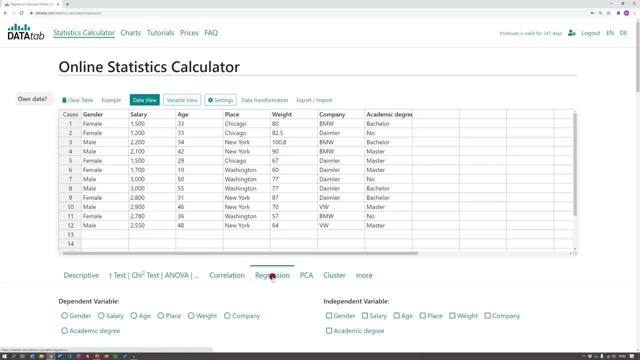 calculate a regression. So we choose the tab regression. On the left side you can select your dependent variables and on the right side your independent variables. Let's say we want to investigate what influences the salary. So we simply click on salary and let's say as: 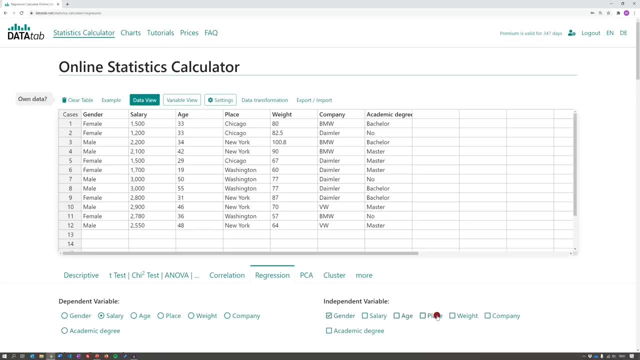 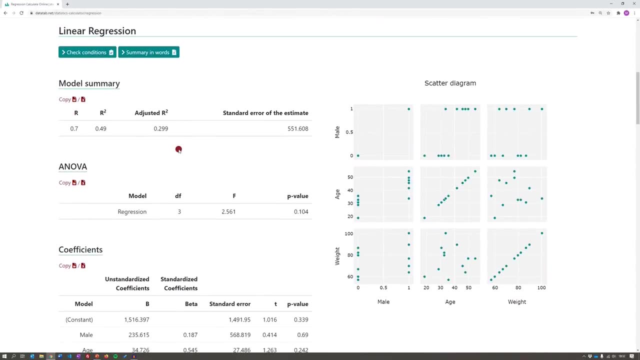 independent variables. we select gender, age and weight. Now, if we scroll down, we already see the results of the linear regression. In the first table we see the model summary. In the second table we see the ANOVA. In the third table we can see. 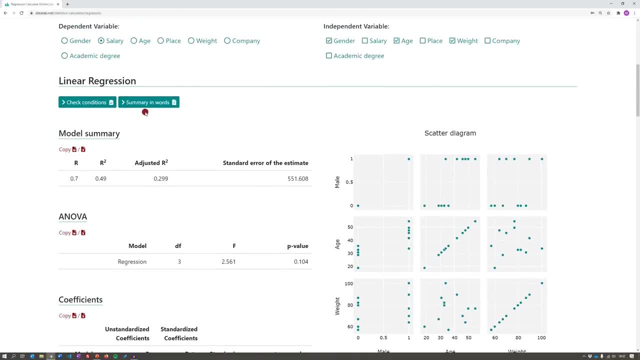 all the results of the linear regression. In the third table we can see all the results of the linear regression. If you like, you can click on summary in words and you get the interpretation of the results. Further, if you want to check the conditions for your regression model, you can click. 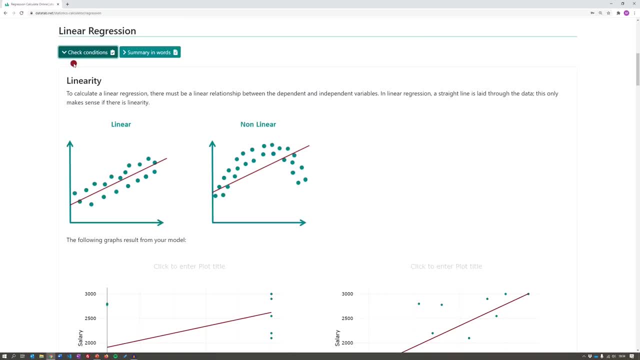 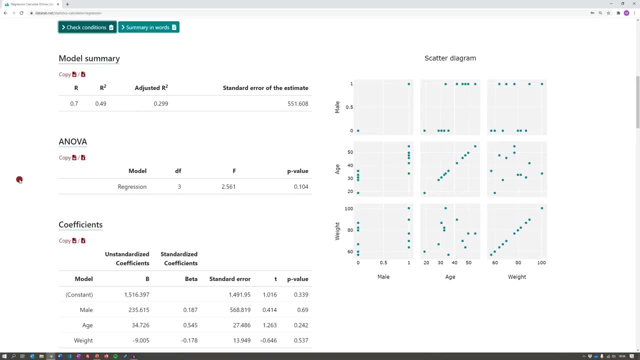 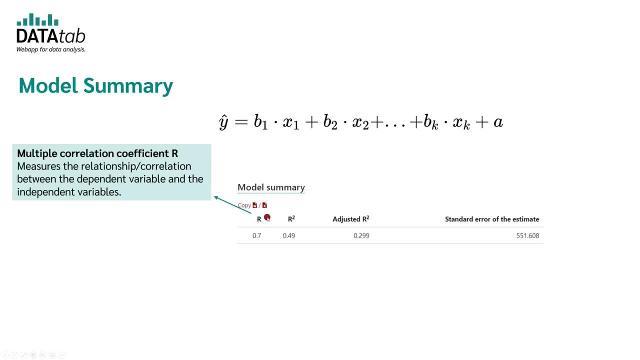 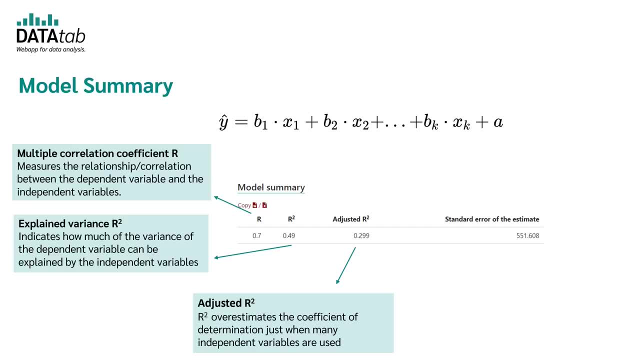 because R-square overestimates the coefficient of the determination when many independent variables are used. And finally, in the model summary, it's important to look at the standard estimation error. The standard estimation error indicates by how much the model overestimates the dependent variable on average. 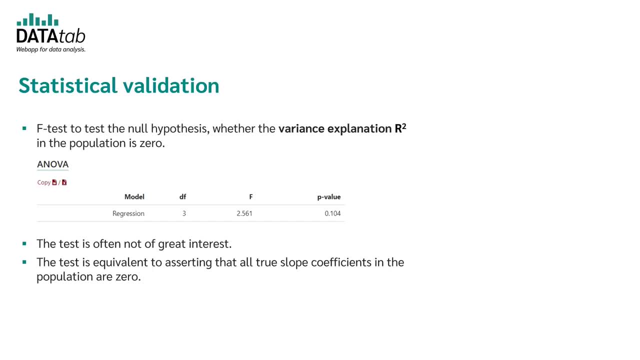 In the second table you find the statistical validation. Here an F-test is provided which tests the null hypothesis whether the variance explanation R-square in the population is zero. In general this test is often not of such a great interest. The test is equivalent to asserting that all slope coefficients in the population are zero. 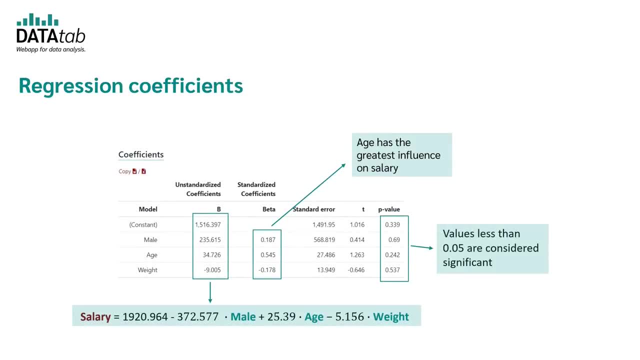 The next table is of great importance because it shows the regression coefficients. The next table is of great importance because it shows the regression coefficients. In this table you find all the independent variables: the unstandardized coefficients b, the standardized coefficients beta, the standard error, the t and the p-value.